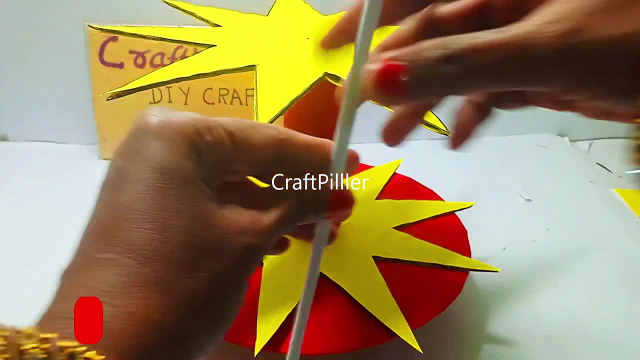 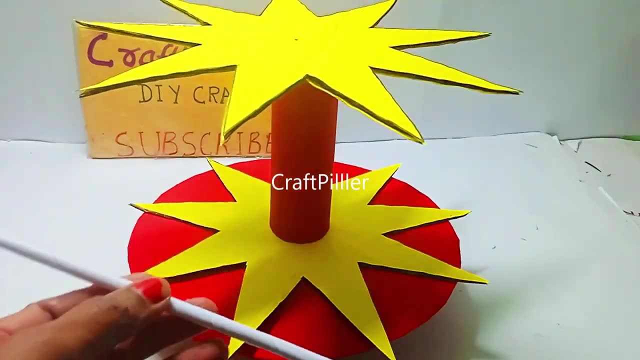 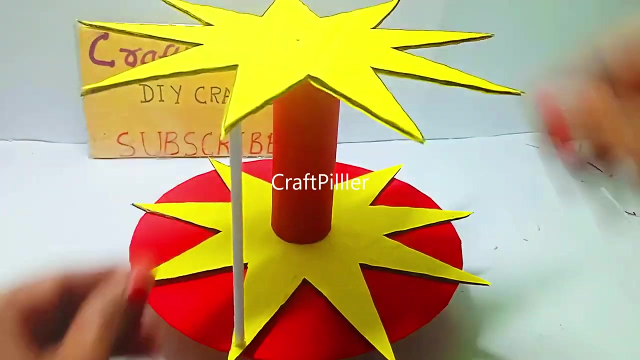 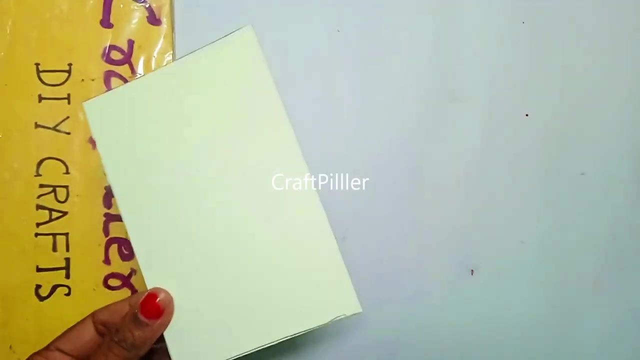 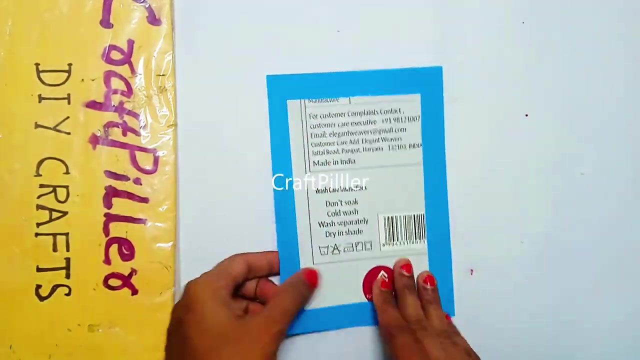 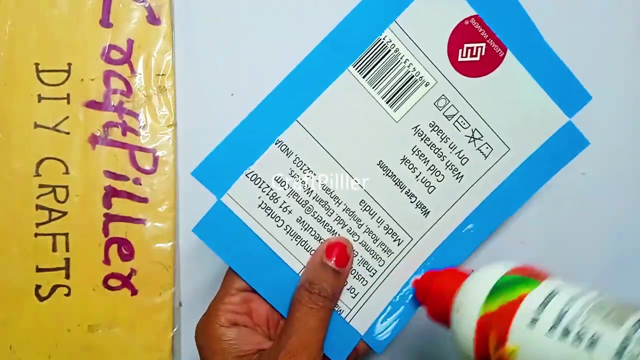 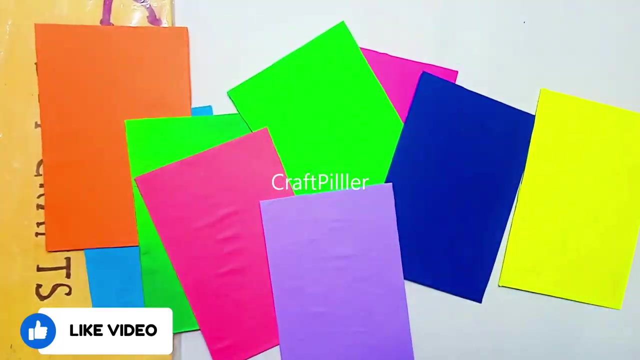 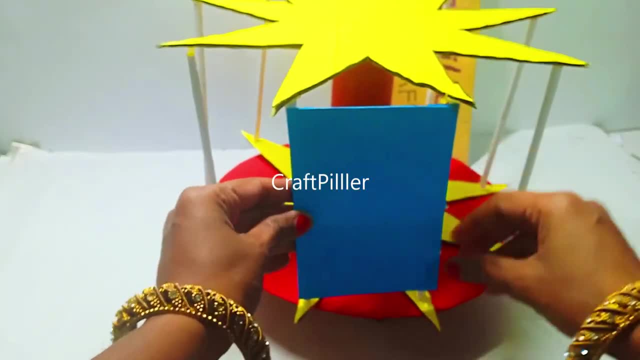 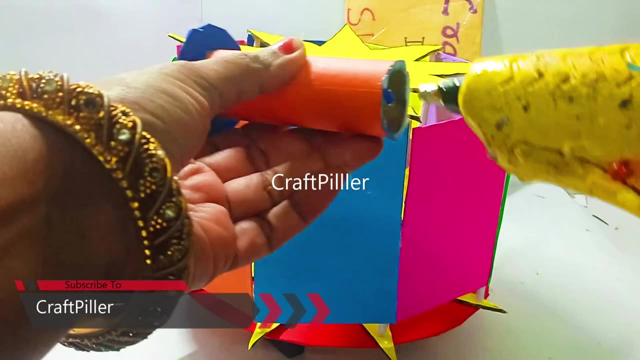 I think I need love. I'm going through hell. I fake like I'm fine, but I know you can't tell. Like nothing, I've found my mind overwhelms. I think that I'm broken, but I know you can't help. I know I'm not perfect. 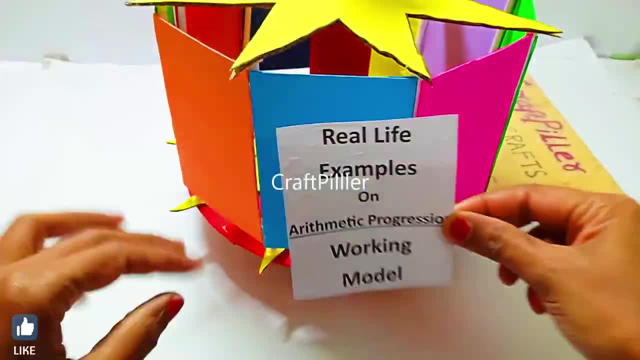 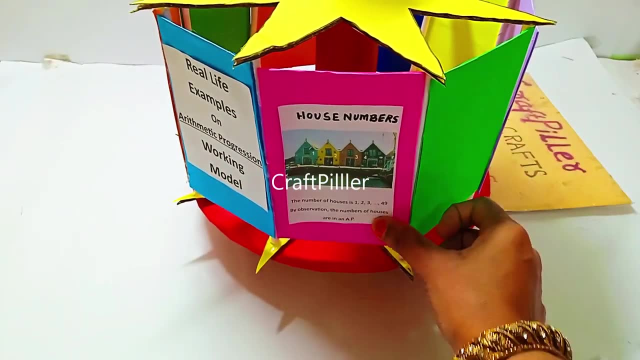 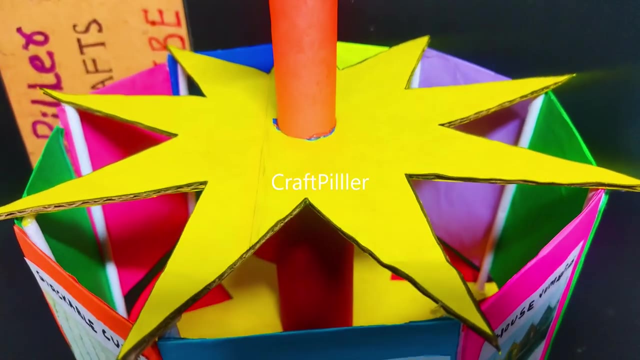 But some days I feel far more worthless. Baby, you make me feel nervous. If I still have you, I have purpose, It's all worth it. I know you told your friend you're not okay And tell me what's wrong and why you never said you felt that way. 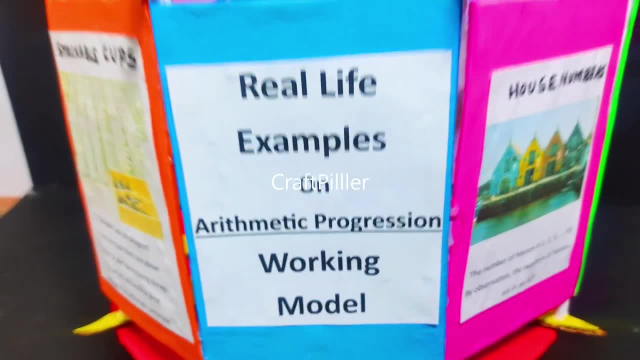 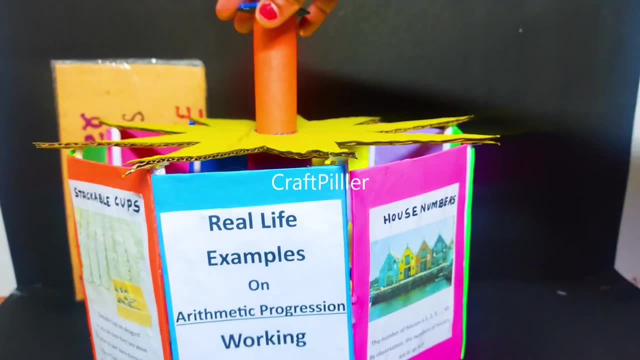 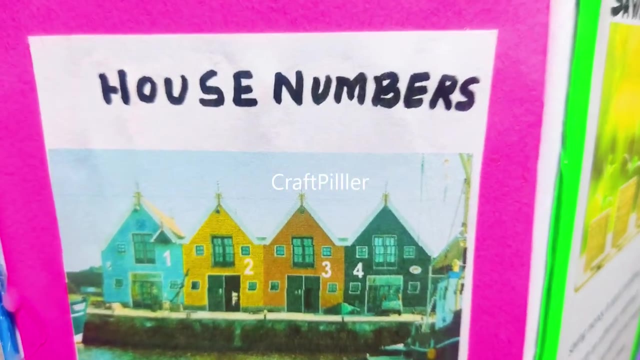 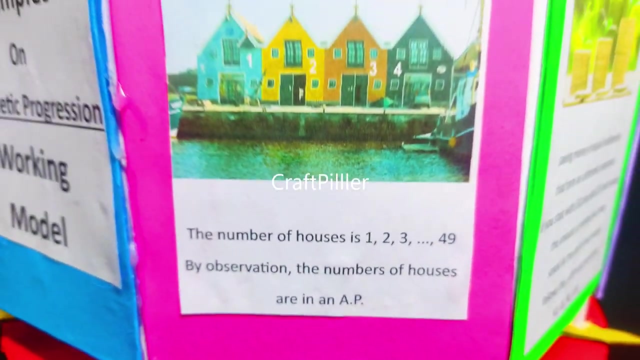 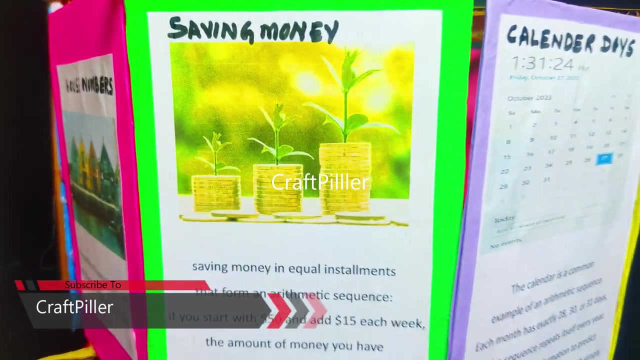 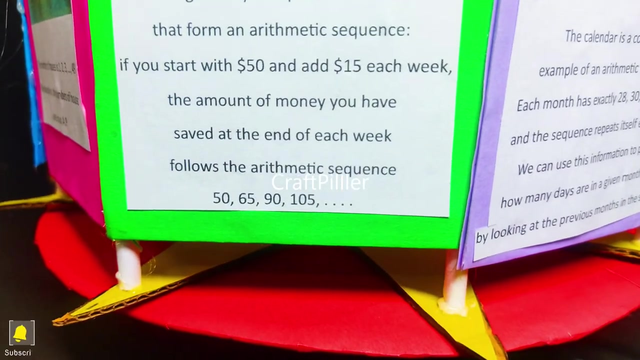 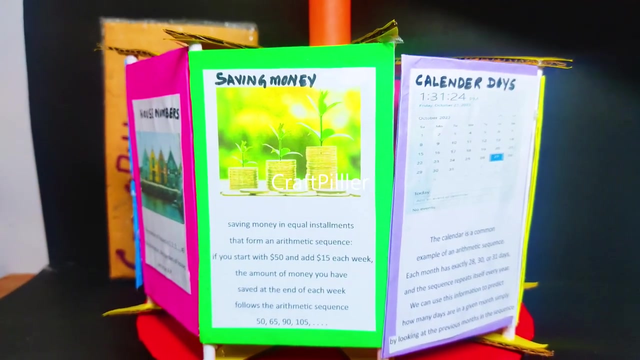 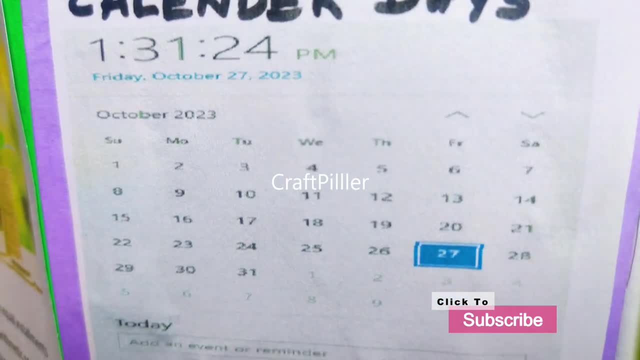 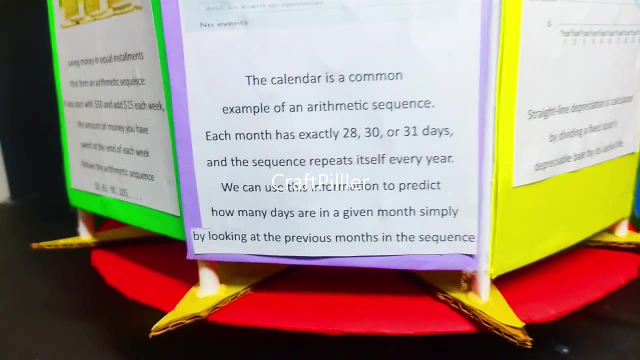 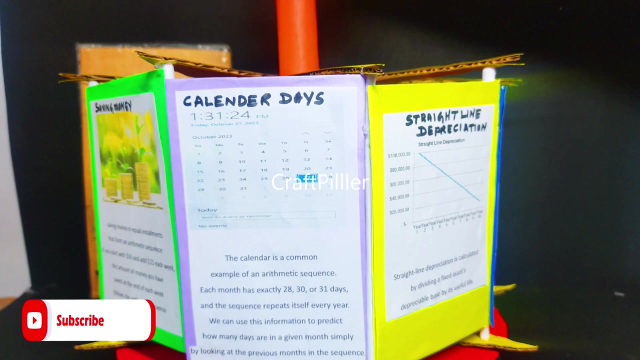 I know you told your friend you're not okay As you fade away. As you fade away And tell me what's wrong and why you never said you felt that way. I guess you're trying to stay strong and fake a smile until I look away, But I've known you too long. it hurts to watch your blue eyes fade to grey.